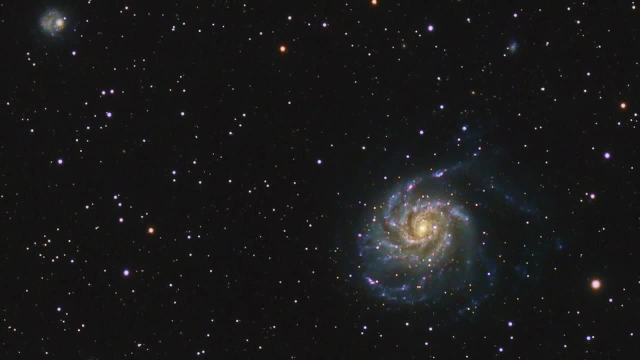 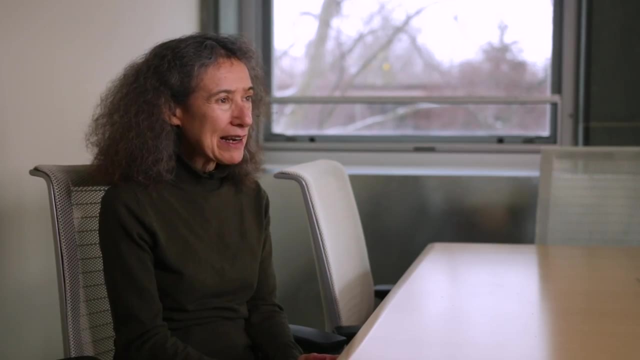 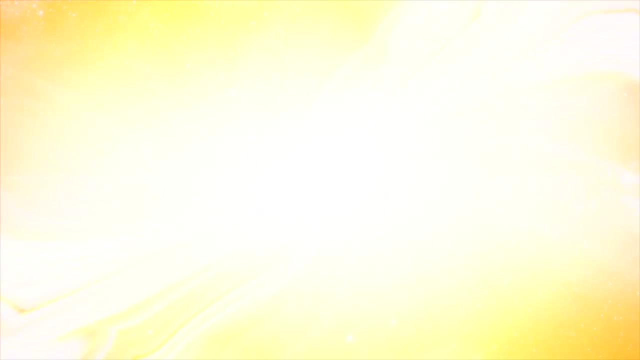 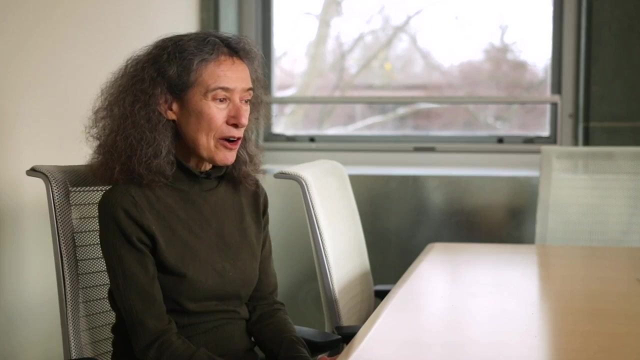 cosmic rays that just defy all our expectations, and I became fascinated, as a young student, with all the physics and mathematics that goes into describing cosmic rays. Cosmic rays are charged particles, mostly protons, that are moving at nearly the speed of light, and in our own galaxy about one particle in a billion is a cosmic ray. 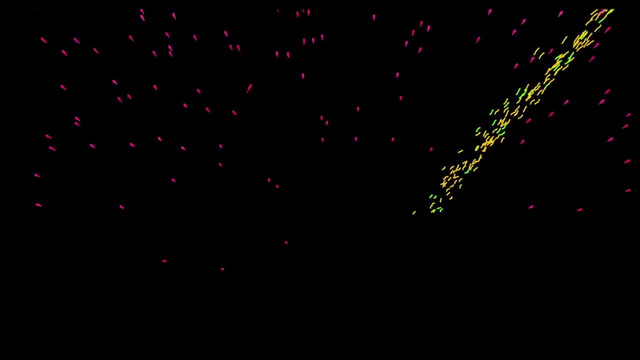 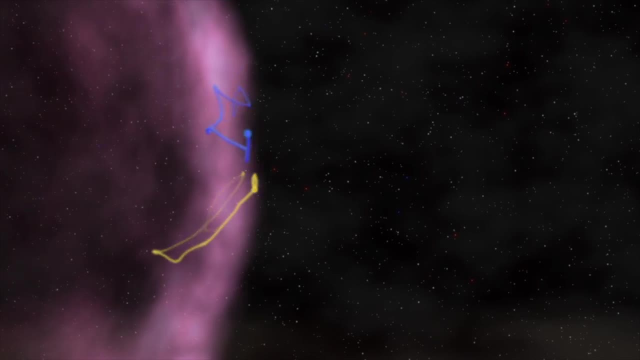 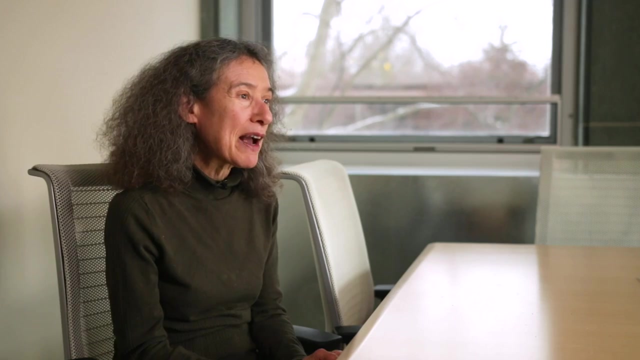 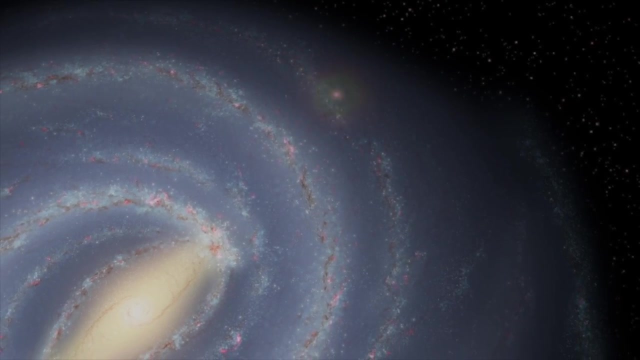 That group of one in a billion particles carries as much energy as all the other particles combined, and if we try to follow each one through its complex motion through the magnetic field, all the computers in the world wouldn't even come close. But by describing the cosmic rays as a fluid we can make the problem solvable. We think that cosmic rays 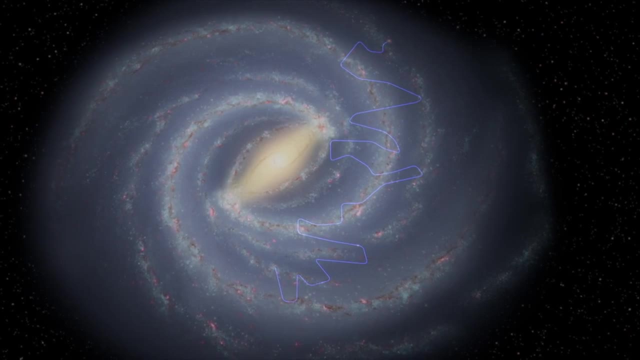 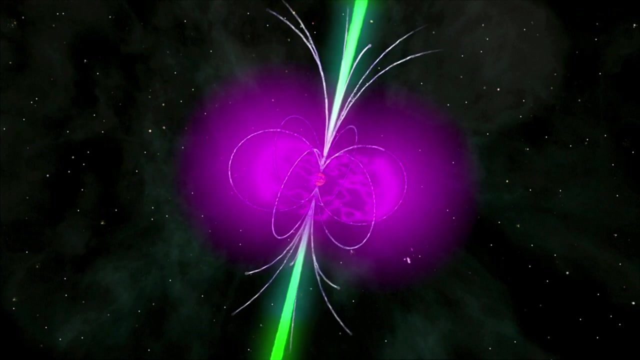 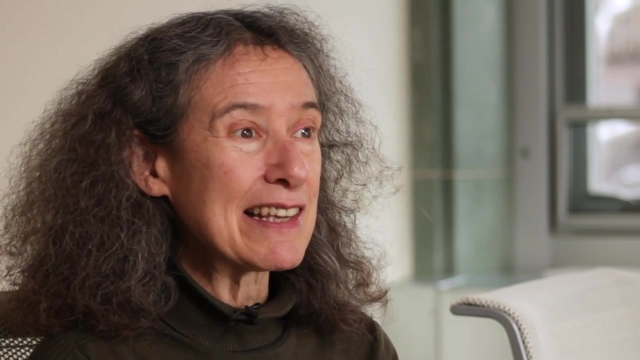 are formed due to an interaction with the magnetic field that the galaxy carries. Although there are magnetic fields in virtually every astrophysical body, we don't know where they came from, And so, by studying magnetic fields in galaxies and trying to detect magnetic fields in very young 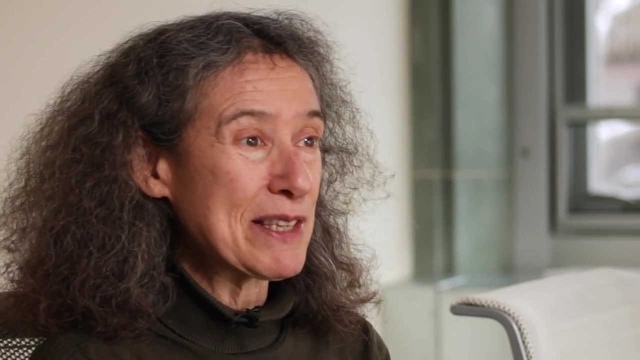 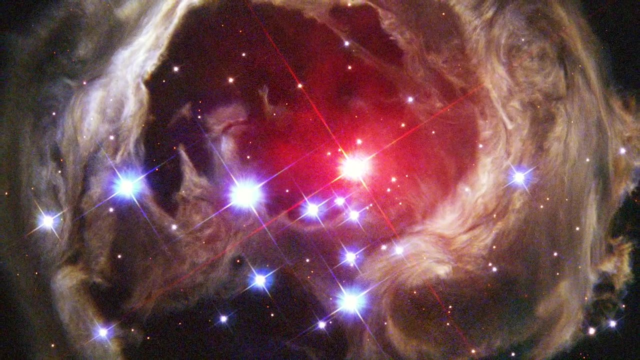 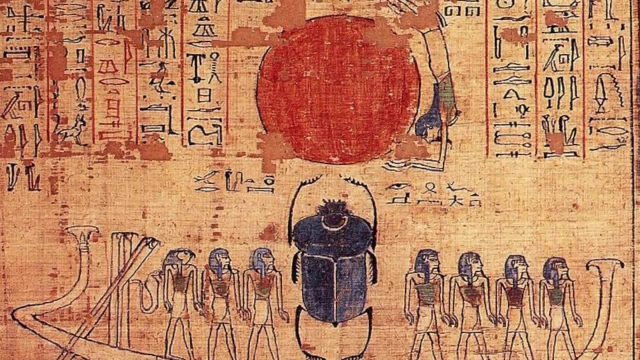 galaxies. we can learn something about this cosmic mystery. Human beings have always wondered what the world is made of. It's part of our culture If you look at any society, any ancient civilization. they've always told stories and they've tried to understand where we came from. 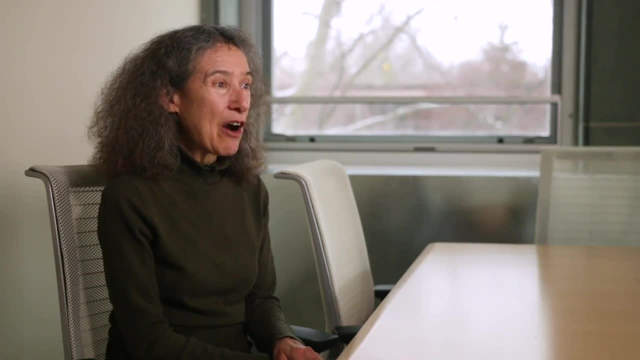 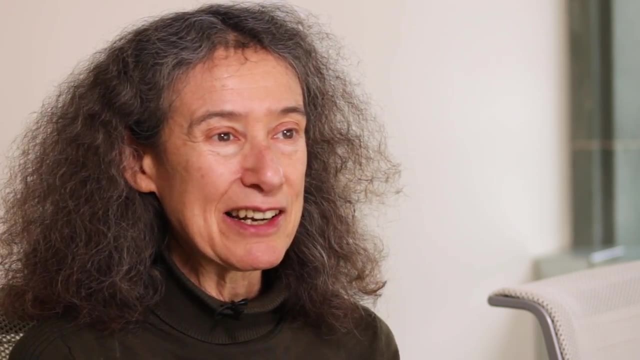 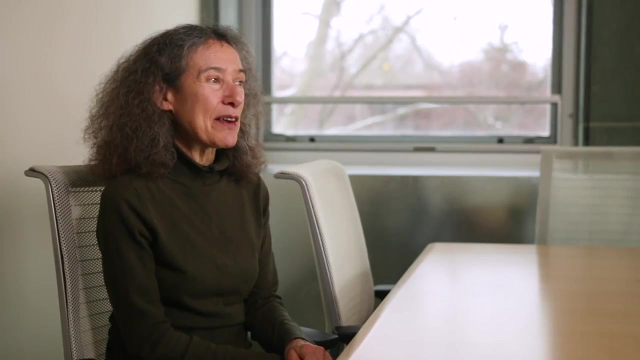 where we're going, And astronomy and astrophysics are the modern take on this. It's now more than half a century that I became interested in astronomy and I've never run out of questions or problems. It satisfies the human quest to discover where we're from.